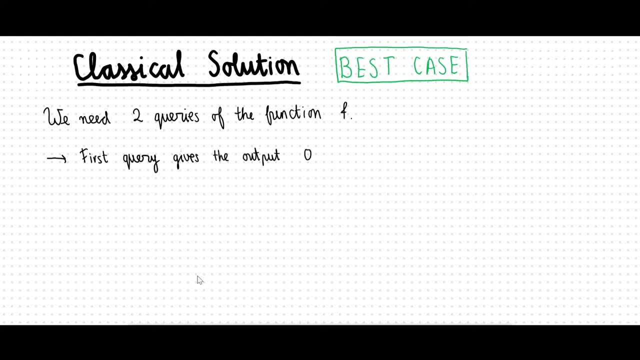 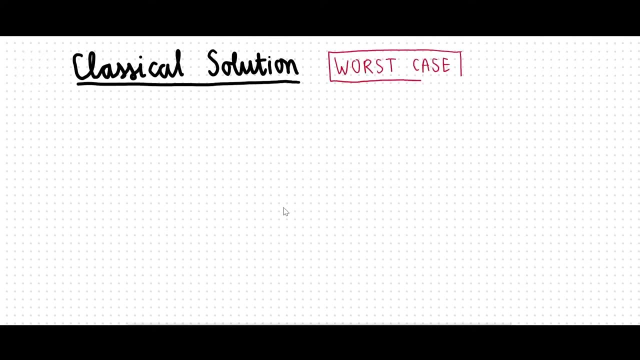 If our first query gives the output 0, and our second query gives the output 1,, then we know for certain that f must be balanced. However, in the worst-case scenario of the classical solution, we need as much as 2 to the power n. 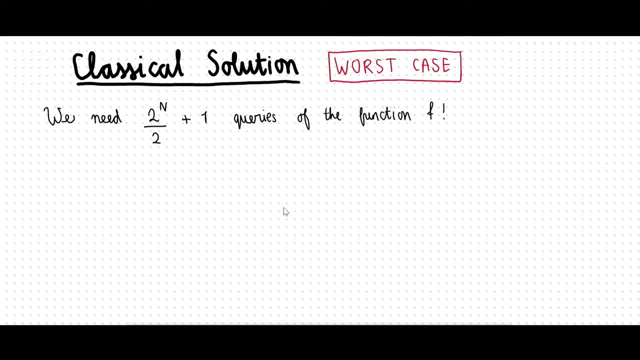 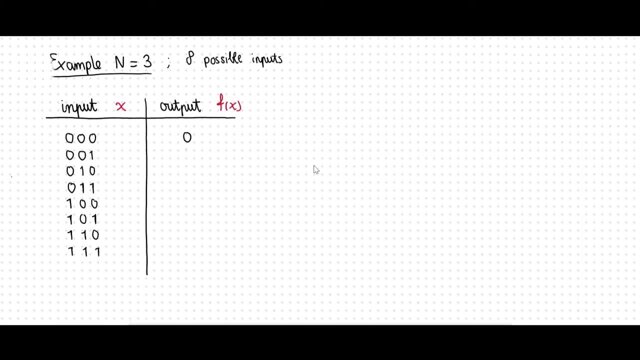 divided by 2, plus 1 queries of the function f. This will be illustrated with an example. Consider the case with 3 bits. Then there are 8 possible inputs to our function f. Let's say we already tried 4 input values. 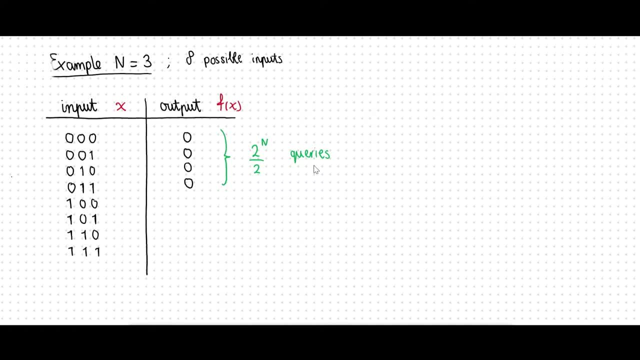 and have received 4 times the output 0. Then we have done 2 to the power n divided by 2 queries of our function. The next query can either give the output 0, from which we can conclude that f must be constant. 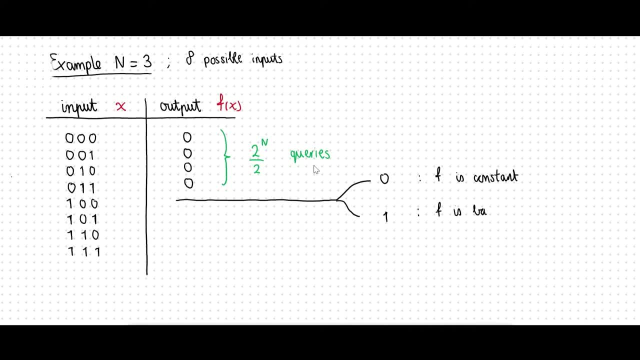 or the output 1, which means f must be balanced. Therefore we need 2 to the power, n divided by 2, plus 1 queries, to be 100% certain whether f is constant or balanced. Now we will go over to the quantum. 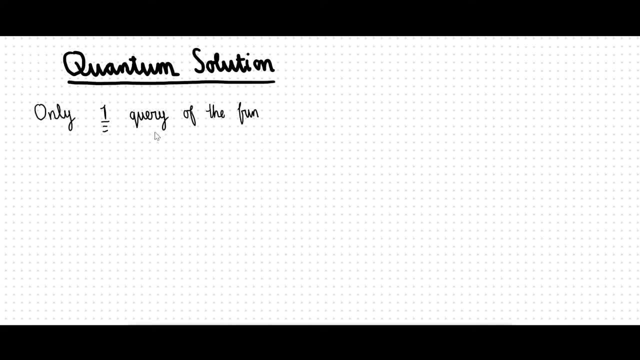 Here only one query of the function f is needed. To this end we need to implement the function f as the quantum oracle that maps the state x- y to the state x- y plus f, where the plus sign means addition modulo 2.. 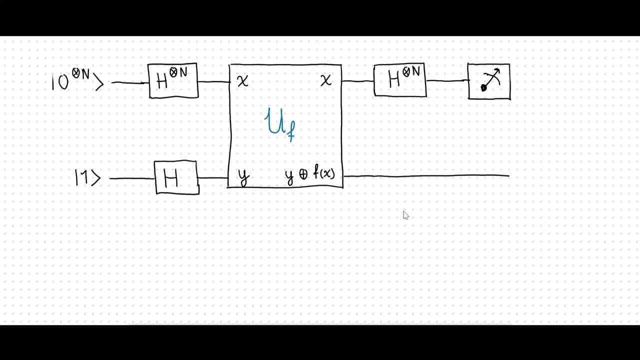 We call this U. The generic circuit can be represented as follows, where we define 4 quantum states: psi 0,, 1,, 2 and 3.. We need an n-qubit register initialized to 0, and an ancilla qubit initialized to 1.. 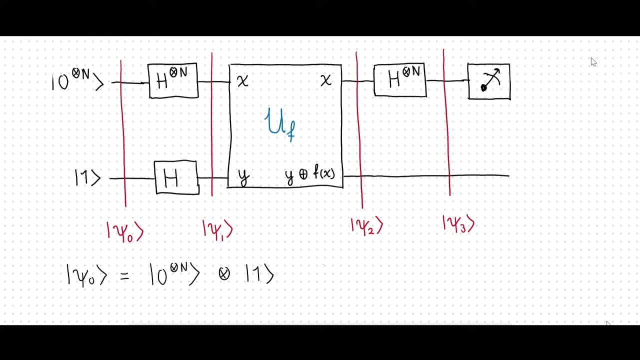 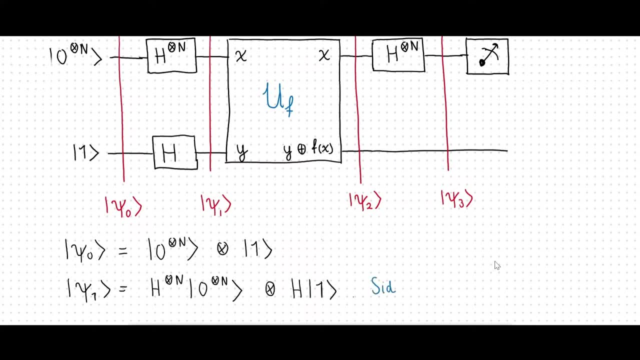 This is psi 0.. For psi 1, we need to apply n Hadamard gates in parallel to the first register, in combination with a Hadamard gate to our ancilla qubit To explain this n-qubit Hadamard transform. 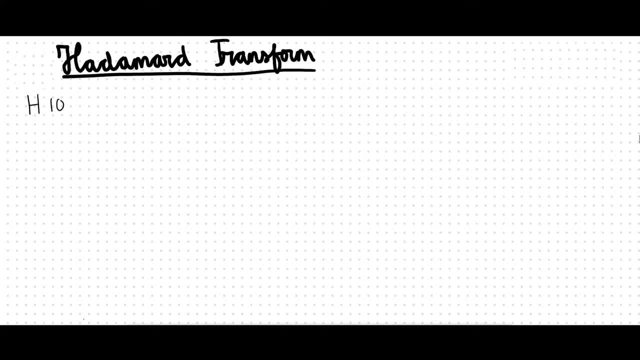 we will take a small sidestep. The Hadamard gate acts on the qubit states 0 and 1 as follows: If we take a 2-qubit state and apply two Hadamard gates in parallel, we can write this as follows: 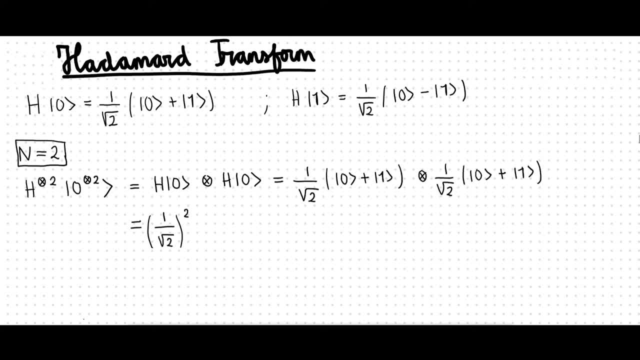 Combining the terms, we get a superposition of the states 0, 0, 0, 1,, 1, 0 and 1, 1.. We can write this using a 2-bit string notation as a superposition of the states 0,, 1,, 2 and 3.. 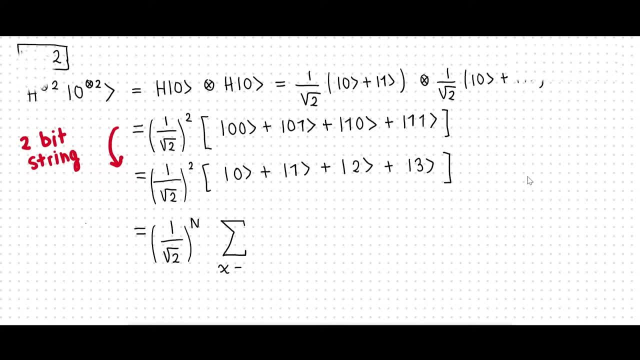 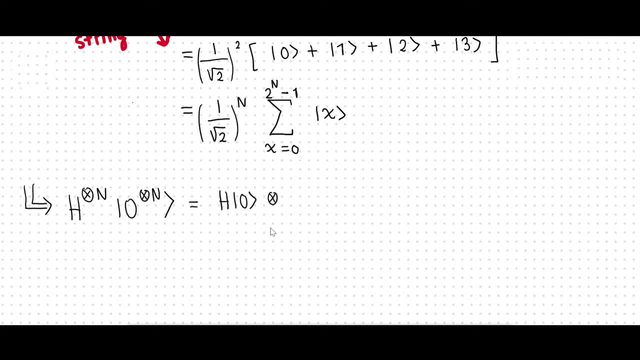 More generally, using the n-bit string notation we can write the action of n Hadamard gates to an n-qubit register in the concise notation of a sum over the state x, from axis 0 to axis 2, to the power n-1,. 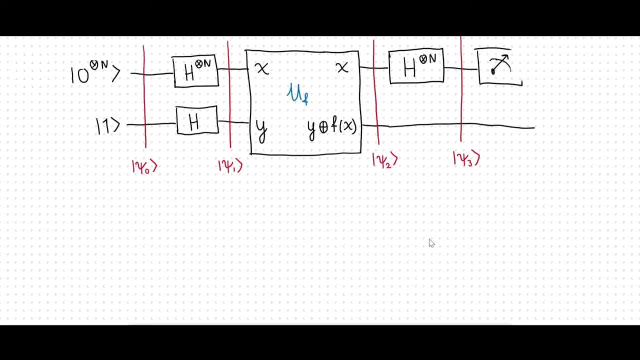 with, of course, a normalization factor. Let's go back to our quantum circuits. Now we know how to write down psi 1, where we of course also apply a Hadamard gate to our ancilla qubit. For psi 2, we need to implement the action of the quantum oracle Uf. 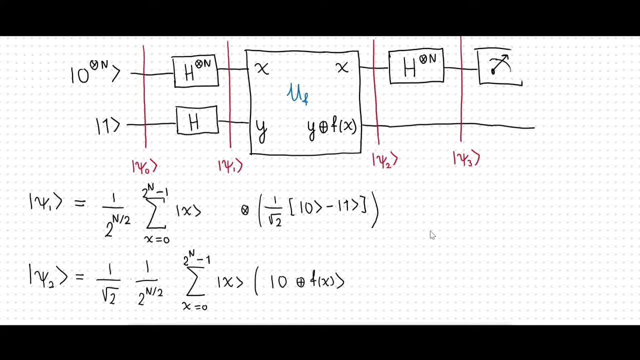 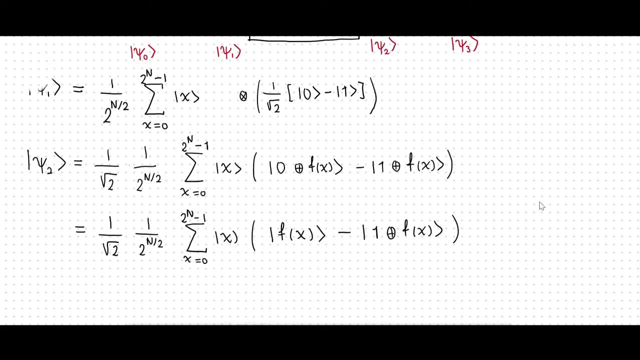 Uf does nothing to our n-qubit register. The state of our ancilla qubit is transformed to 0 plus f, minus 1 plus f. Simplifying, we get this: As f is either 0 or 1, the state of our ancilla qubit is either 0 minus 1 if f is 0,. 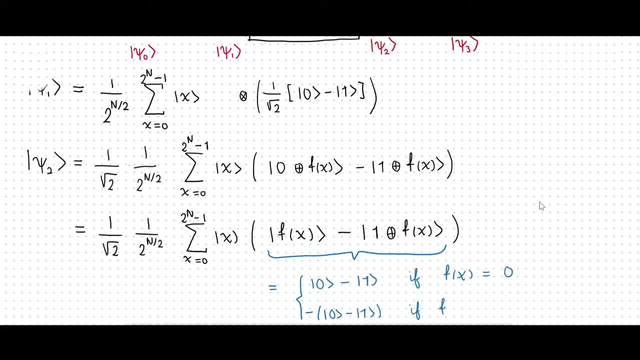 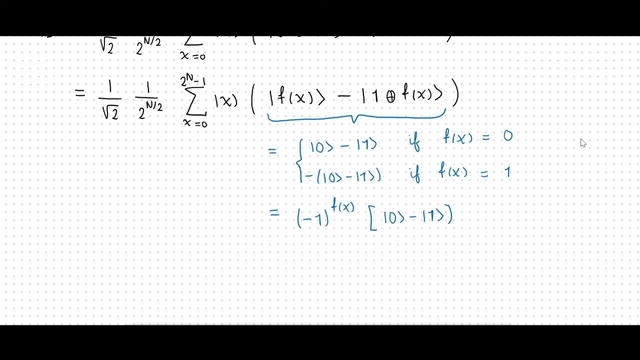 or minus 0 minus 1, if f is 1.. We can also write this as minus 1 to the power f times 0 minus 1.. Therefore, our quantum state, psi 2, can be written down as follows: For psi 3, we need to apply n Hadamard gates in parallel to our first n-qubit register. 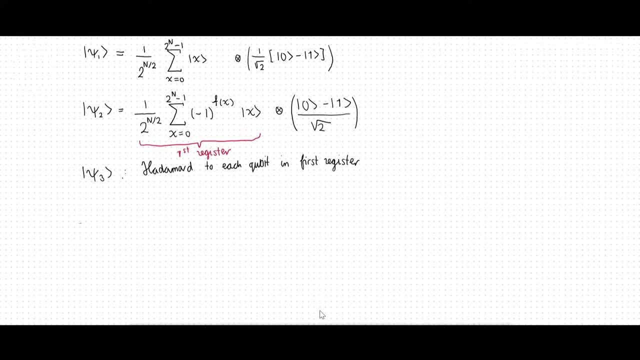 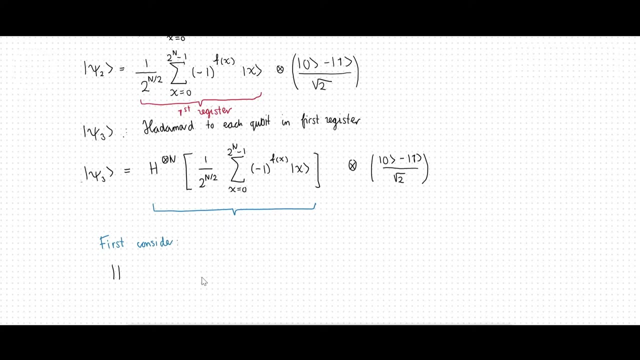 We can for now ignore the second register. To explain how this works, we will first consider how to write down the action of n Hadamard gates to the state x without the sum. This can be written as a sum over y containing an x dot y. 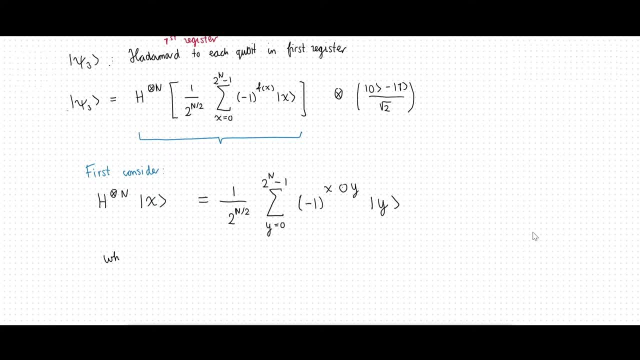 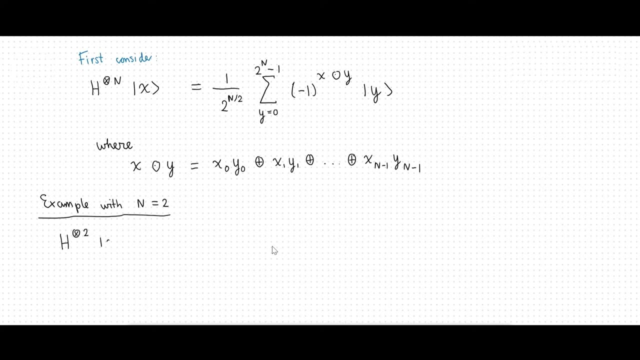 which means the modulo 2 scalar product where we get x0, y0, addition modulo 2, x1, y1, until xn-1, yn-1.. Let's consider an example with n as 2.. An x can either be 0,. 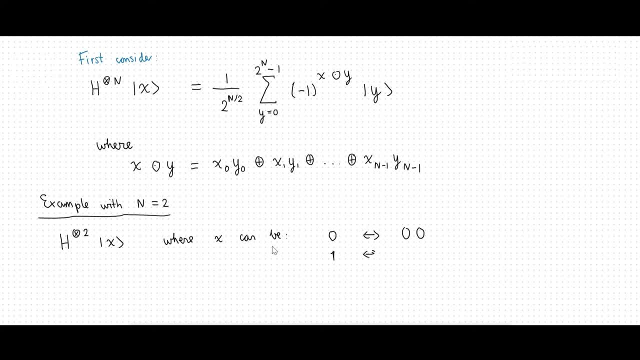 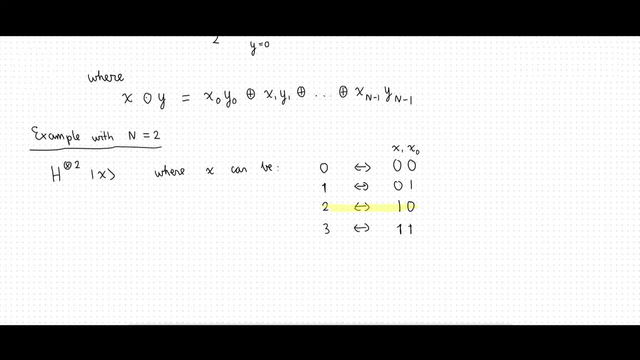 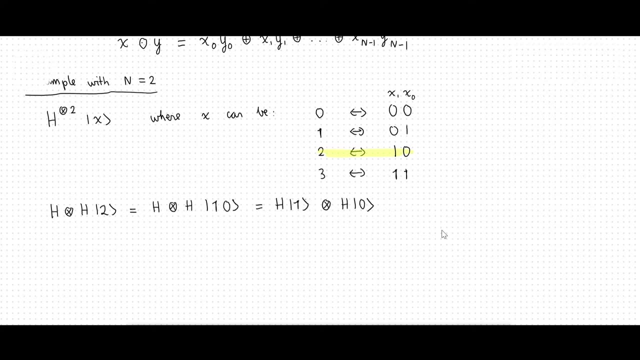 corresponding to the state, 1, corresponding to, 2, corresponding to and 3, corresponding to. We will take x as 2.. Then the two Hadamard gates act on the state as follows: We get again a superposition of the terms and. 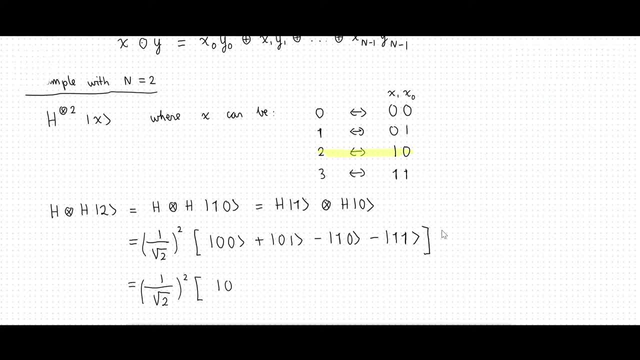 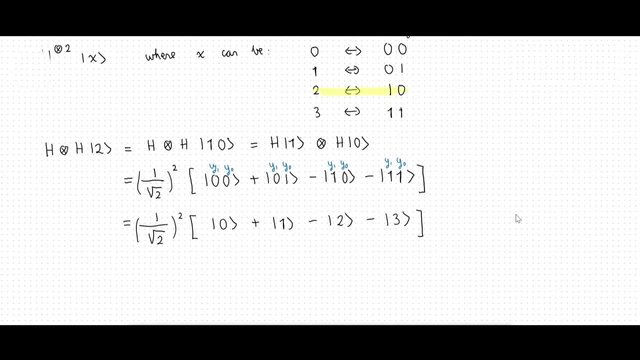 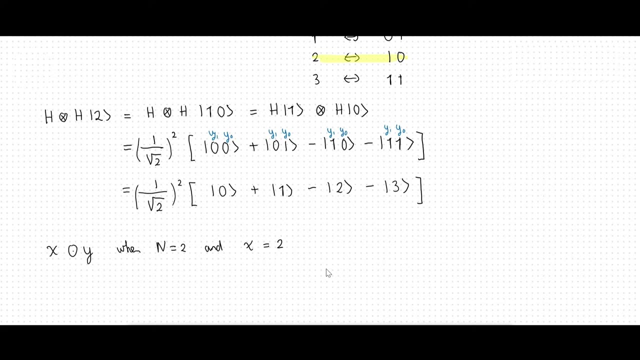 which we can again rewrite using the 2-bit string notation. On the other hand, x dot y, when n is 2 and x is 2, is given as follows: x0 is 0 and x1 is 1.. Therefore, we can write this in our example. 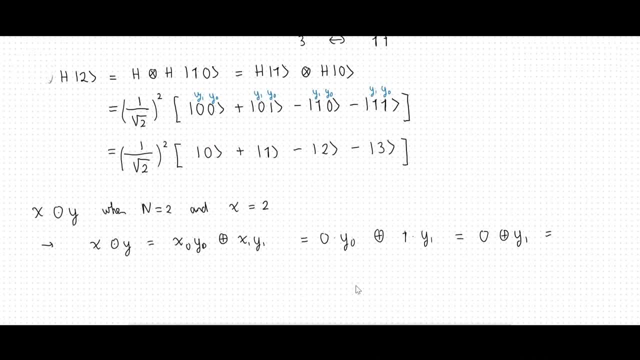 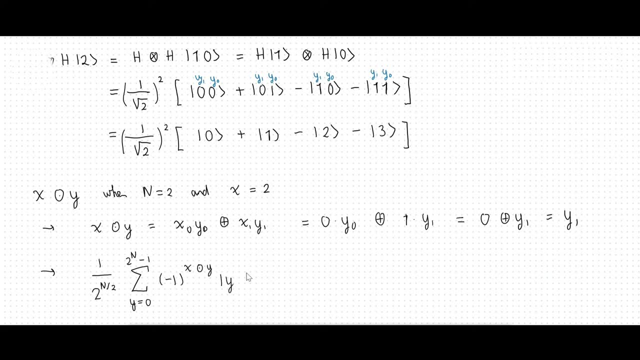 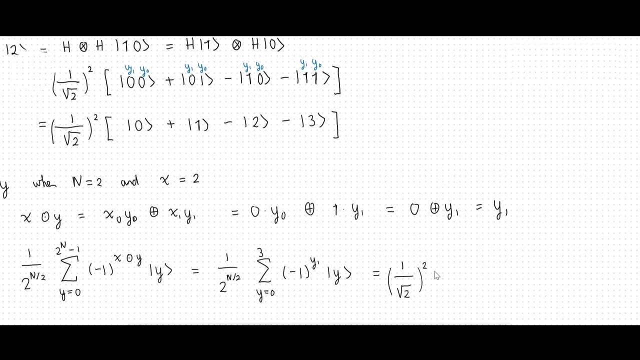 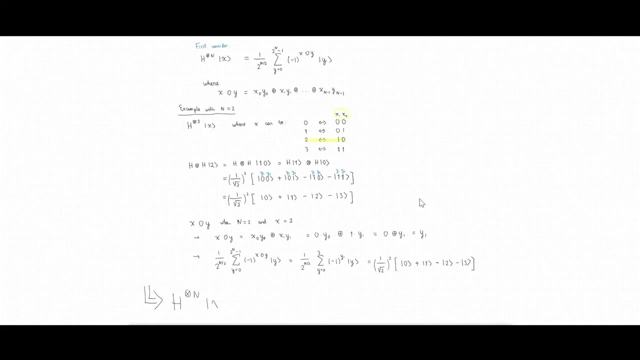 as 0 addition modulo 2, y1, which just equals y1. Therefore, the sum over y just presented can be simplified to this sum. If we write this down, we get exactly the same state we have just derived. Therefore, n Hadamard gates to an n-bit state, x. 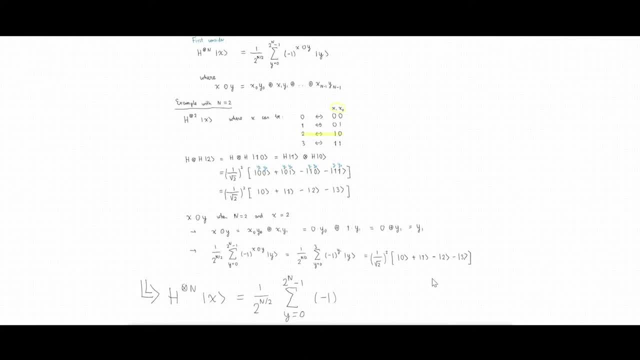 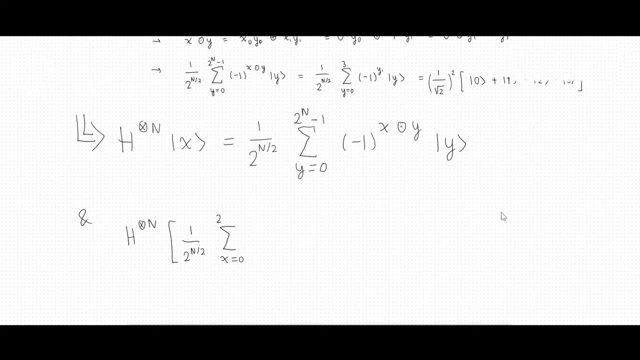 can be written in the concise way as: the sum over y of minus 1 to the power x dot y times the state y. The n-bit Hadamard transform to the sum of the n-bit state x is written down as follows: Simplifying this gives a sum over x. 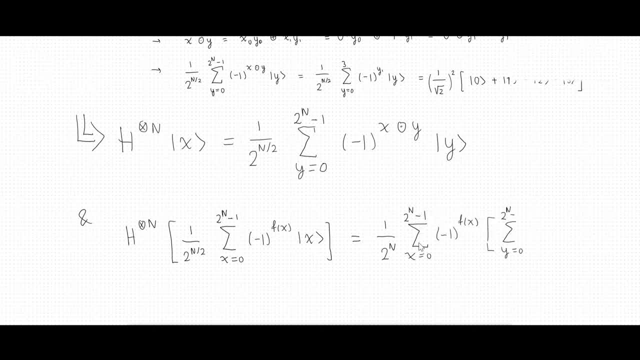 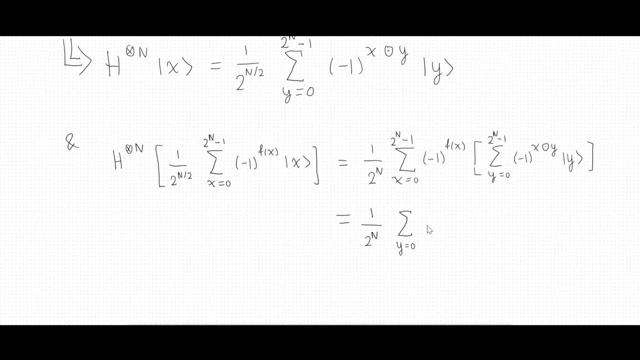 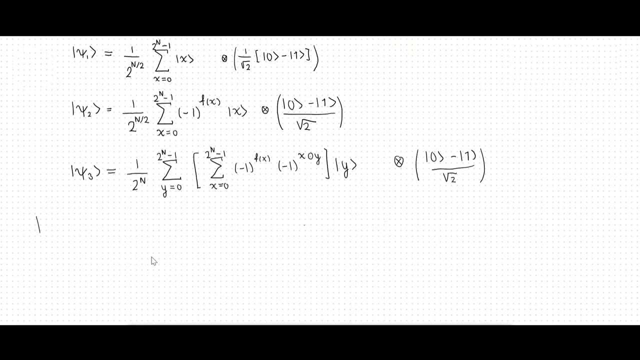 containing the minus 1 to the power of f and a sum over y containing the x dot, y and the state y. Reordering the sums gives us the following final state: psi. Now we know what psi is. we are going to measure the first qubit register. 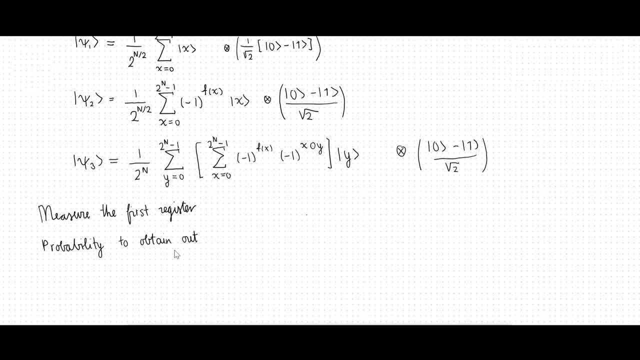 The probability to obtain the outcome y is 0, meaning n qubits in state 0, is given by the amplitude squared of the state y is 0. If we fill in y is 0 to this amplitude, we get this. This can be simplified to this state.